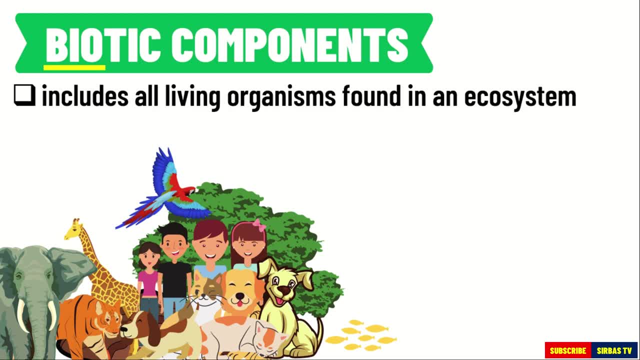 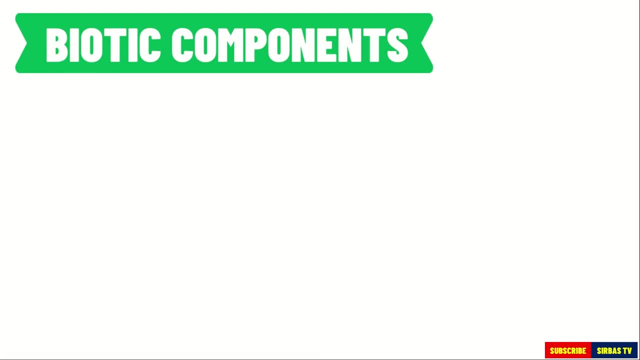 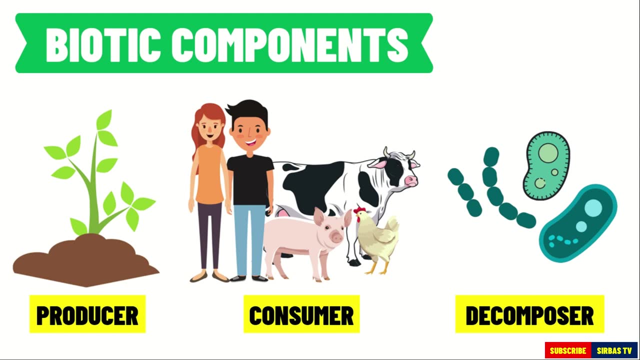 Biotic components of an ecosystem includes all living organisms found in an ecosystem. Biotic components include producer or the plants, consumers, such as animals, and decomposers, such as bacteria. We are going to discuss in detail the role of producers- consumers. 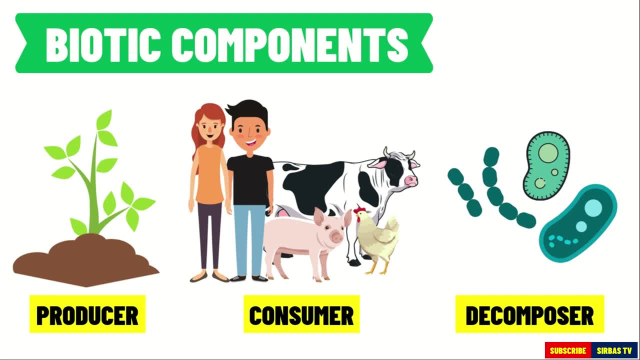 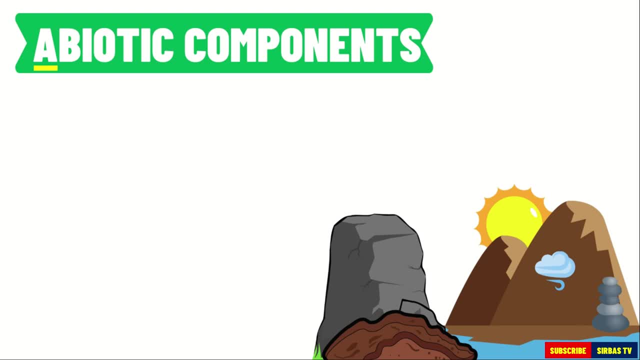 and decomposers in our next video. Let us now talk about the abiotic components of an ecosystem. The word a in the word abiotic means without and the word bio means life. Therefore, abiotic means without life. The abiotic components are the nonliving components or the physical and chemical aspect of an 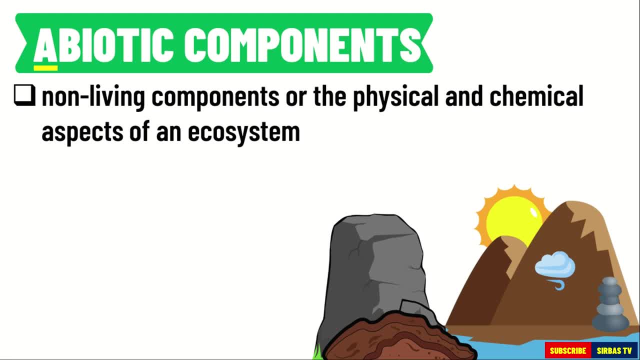 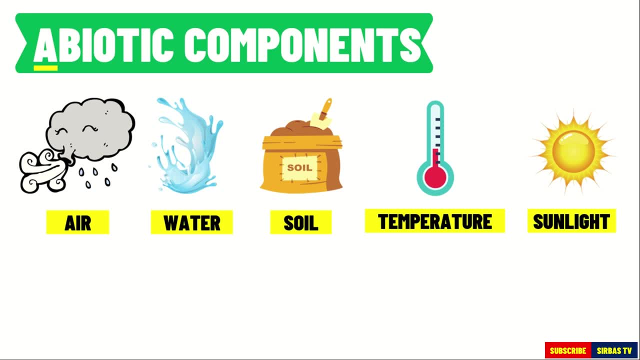 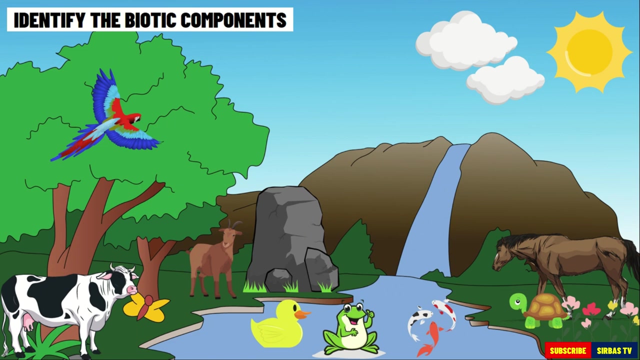 ecosystem. Example of abiotic component components include air, water, soil, temperature and sunlight. These abiotic components have important roles in the survival of living organisms in an ecosystem. Take a look at this picture. What are the different biotic components that can you identify? 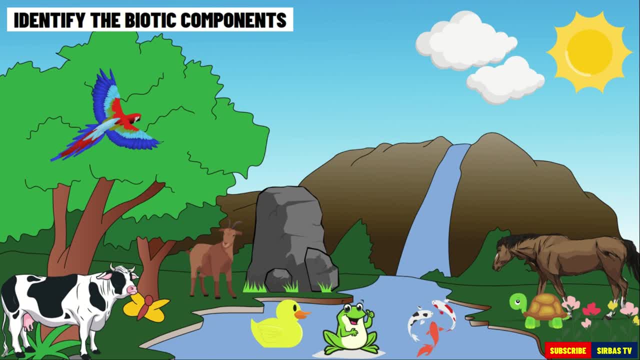 Correct. The biotic components in this ecosystem are the following: Trees, flowers, frog, fish, bird, cow, goat, horse, turtle, bird, duck and butterfly. How about the abiotic components? You are right. The abiotic components are the following: The sunlight clouds. 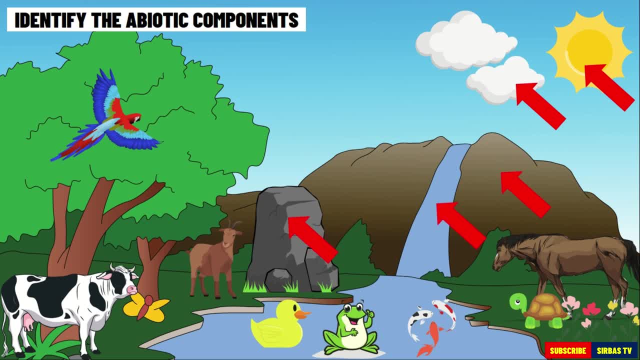 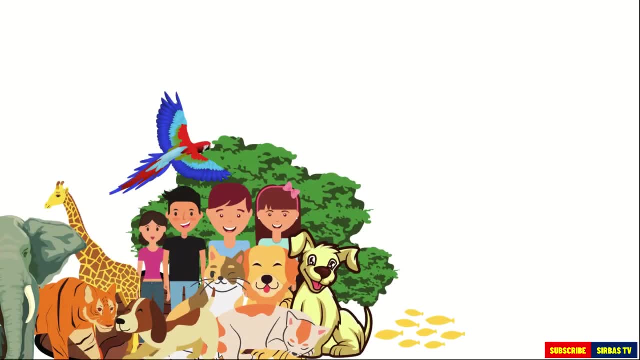 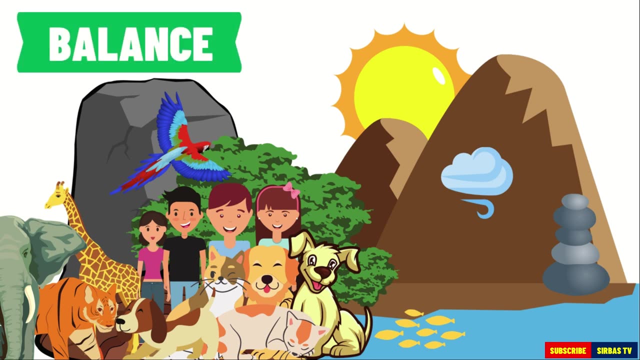 water, mountains, rocks, soil, air and temperature. The biotic and abiotic components of an ecosystem work hand-in-hand and interact with each other to maintain balance in our environment. Without the abiotic components, living things cannot survive- Organisms both. 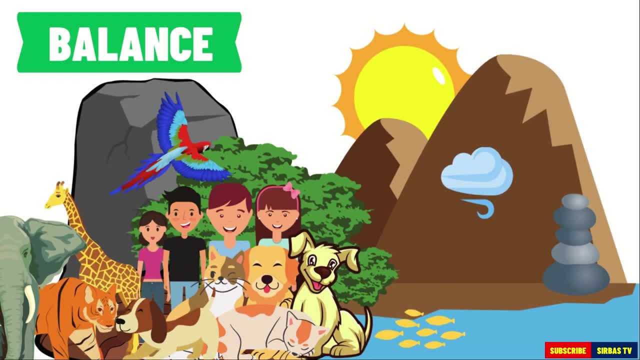 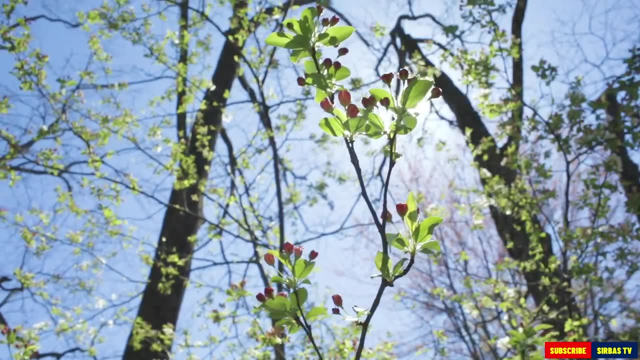 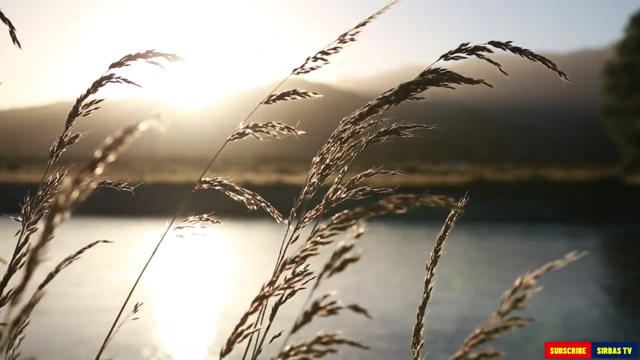 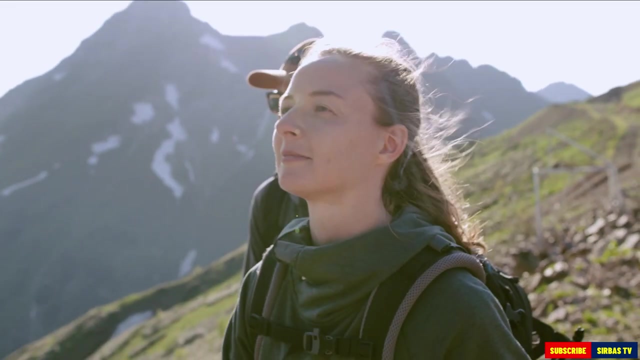 depend on the biotic and abiotic factors in their environment. The light coming from the sun is important to plants for them to make their own food through the process called photosynthesis. The sun plays an important role in the production of oxygen. Air contains oxygen that is produced by plants and trees, which allows animals to